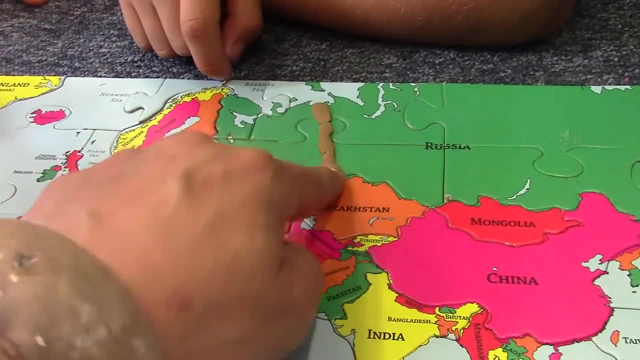 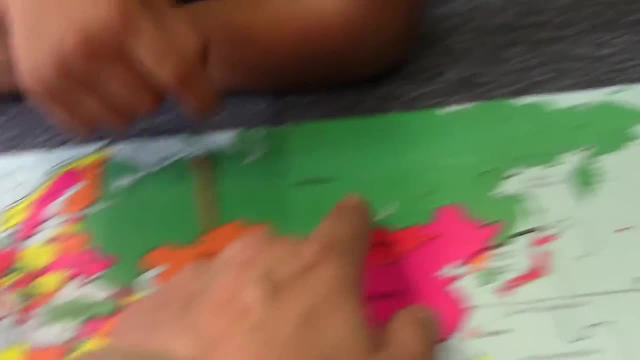 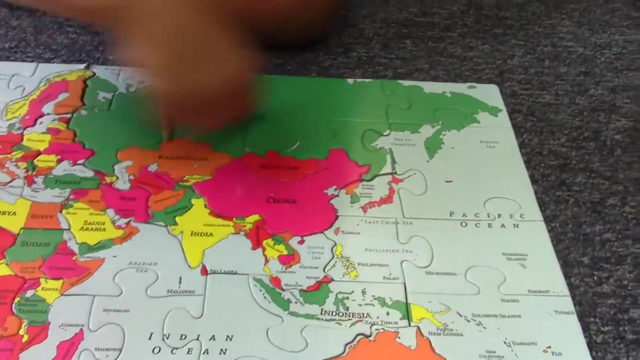 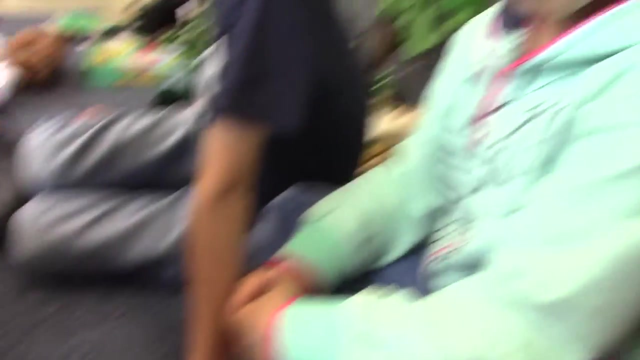 Yes, Between a border, hranice, mountains Mountain is a border between Europe and Asia. So this is Asia. Is this Asia? Where is Japan? Here is Japan. Here is Japan, Japan. Do we have someone here from Japan? Is someone here from Japan, Professor, are you from Japan? 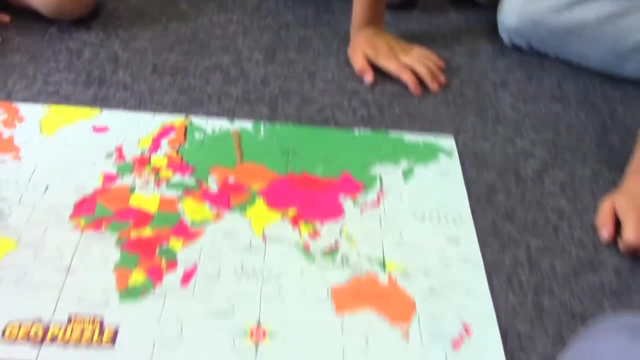 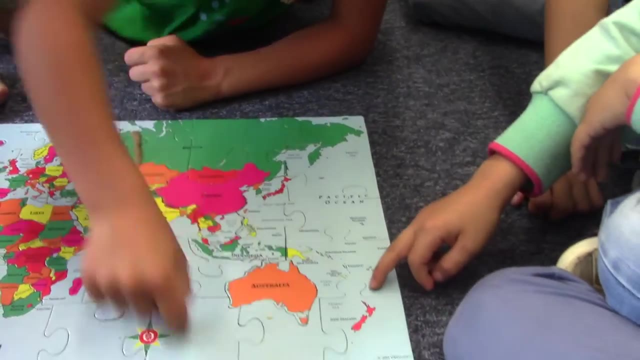 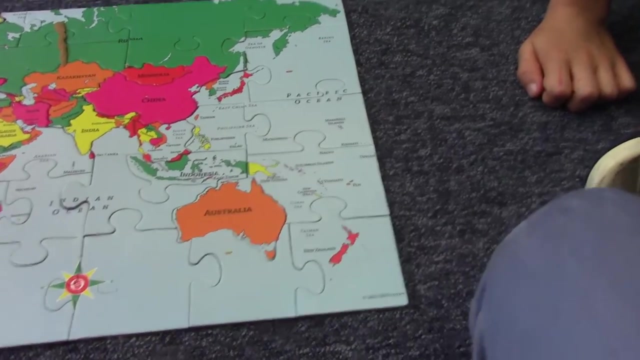 Yes, I see. Okay, Professors, where is Australia? Where is Australia? Here is Australia. Here is Australia. Australasia And New Zealand, And New Zealand And New Zealand. So Australasia is, tell me, if I'm right, Australasia is Australia and New Zealand. 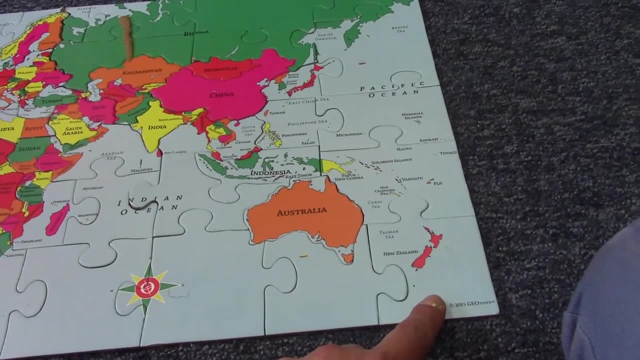 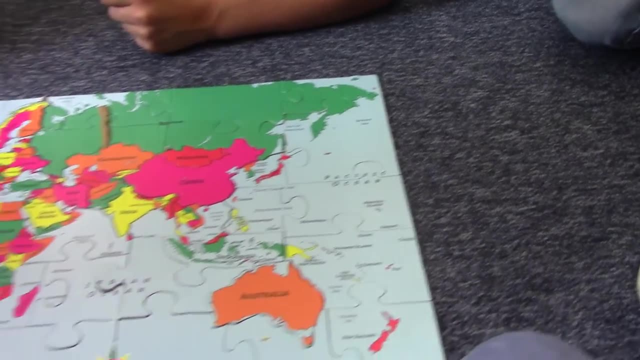 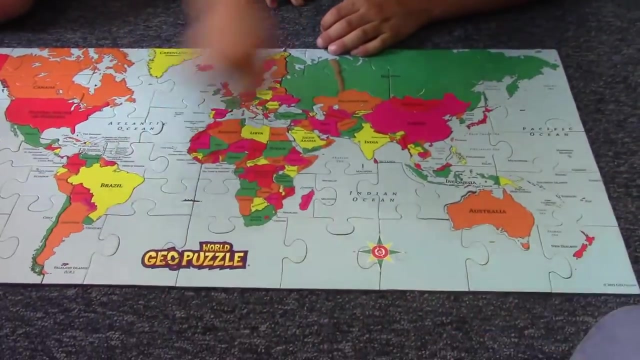 It's Australia and New Zealand. Yes, Yes, Yes, And also this New Guinea. Yes, Yes, I see Where is Antarctica Here, Here. Here is Antarctica. So is Antarctica on this map? No, No, No. 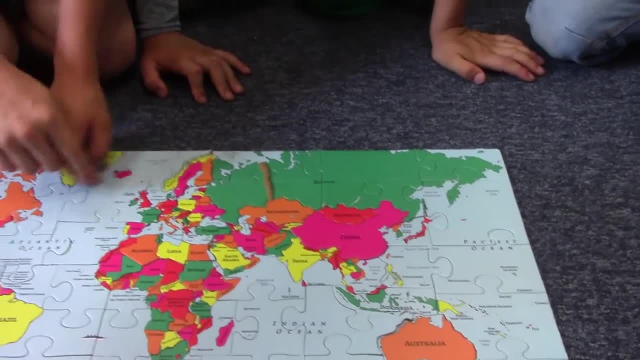 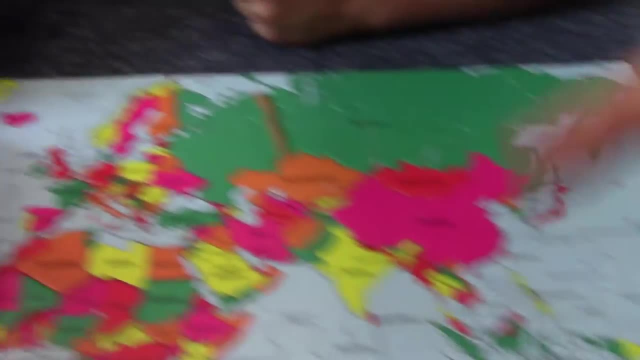 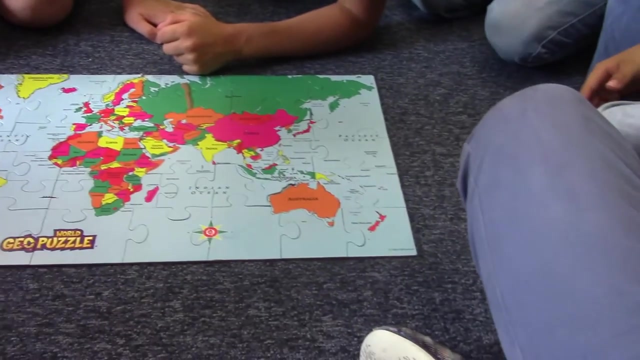 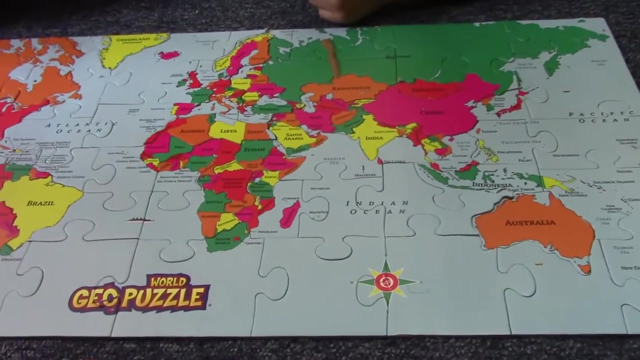 Where is the North Pole Here, Here, But it's not really on the map, is it? No, okay, where is Greenland? very good, thank you so much. don't speak in Czech, okay, so thank you very much for helping me to learn the world. the world, what does? 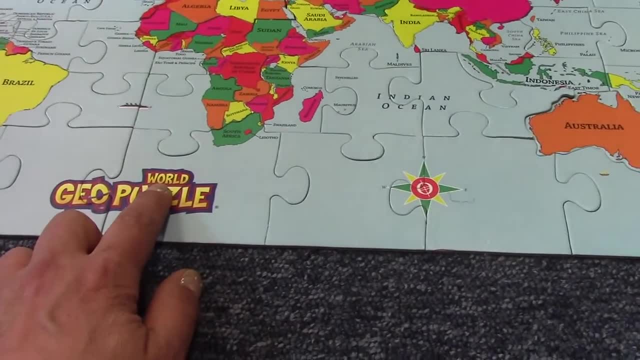 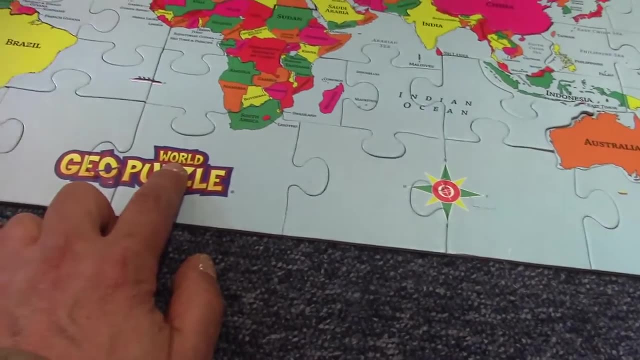 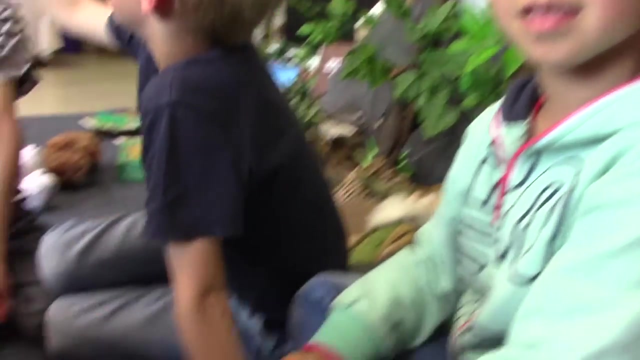 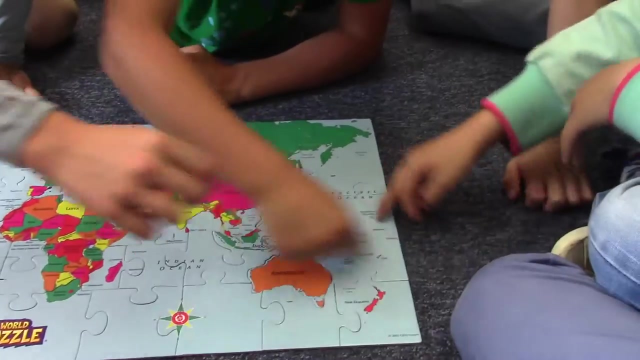 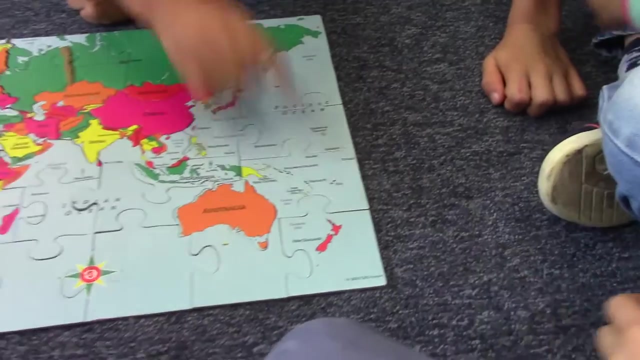 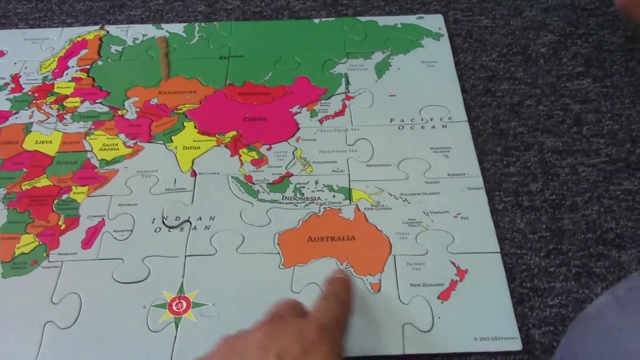 world mean. what does world mean? talk about a professor, Killian, give world. it means, yeah, yeah, so is this a world puzzle from Japan, professor? are you from Japan? yeah, I see, okay, professors, where is Australia? where is Australia? Australia so Australasia is- tell me, if I'm right, Oster Australasia is Australia and New 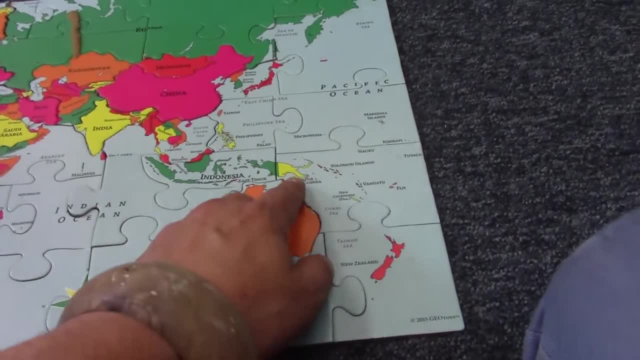 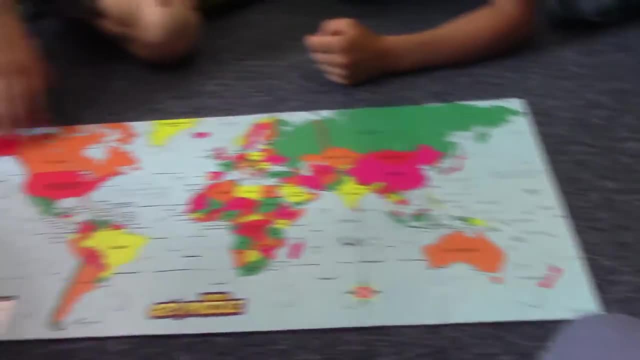 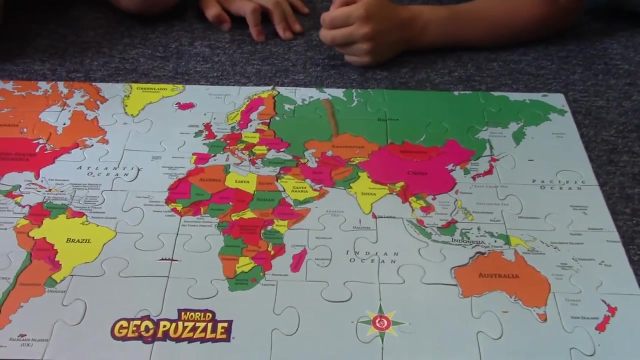 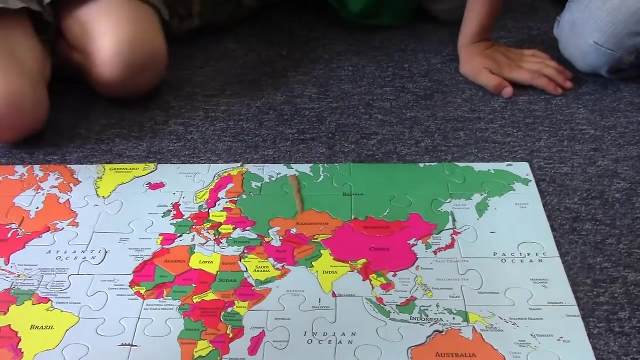 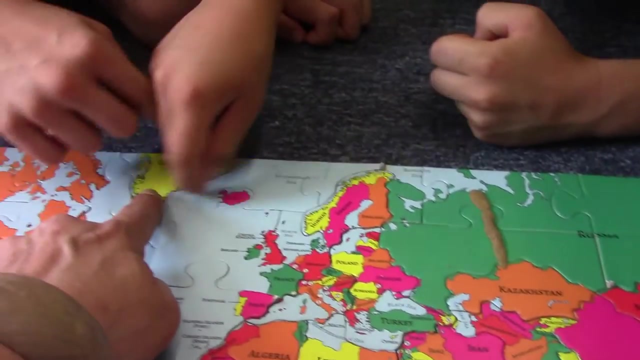 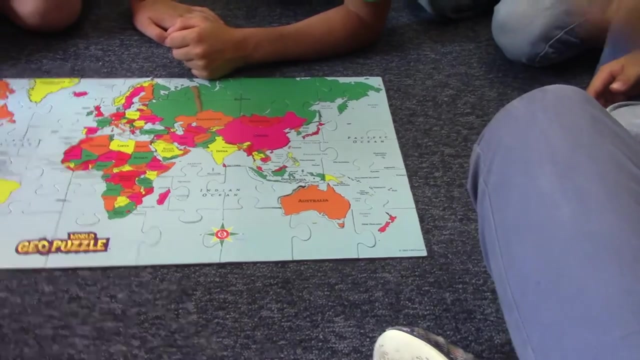 Zealand, yes, yes, and also this New Guinea. yes, I see. where is Antarctica? here is Antarctica. so is Antarctica on this map? where is the North Pole? yeah, Kitaball, yeah, but it's not really on the map, is it okay? where is Greenland? here is Greenland, very good. thank you so much. yeah, yeah z sevnicevich. 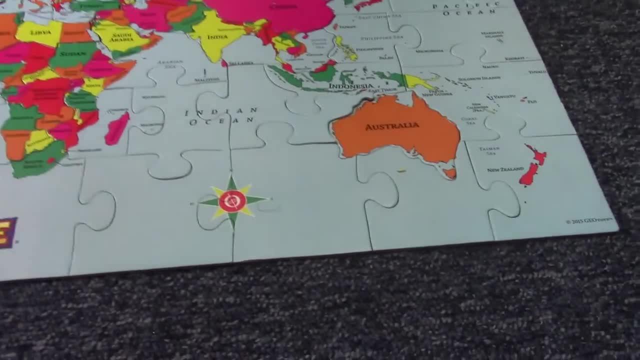 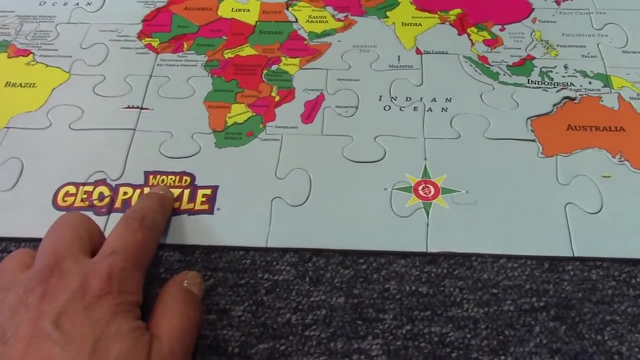 don't speak in Czech, okay, so thank you very much for helping me to learn the world, the world. what does world mean? youpl zyka. what does world mean? tę inclusenko? appreciate that. thanks so much. I appreciate that. thanks for taking the time with us. 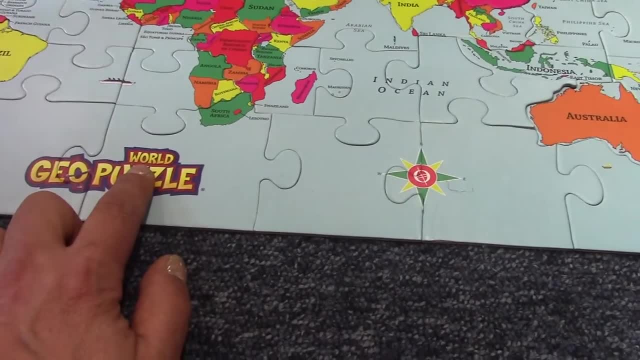 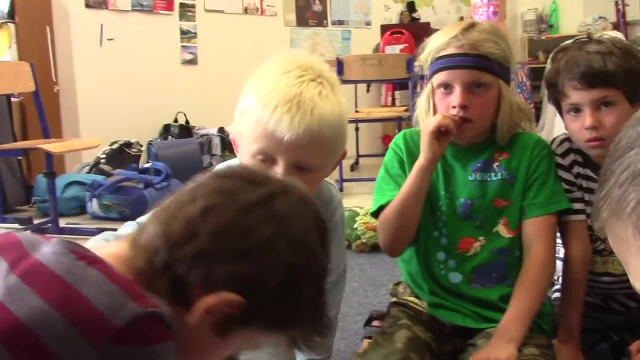 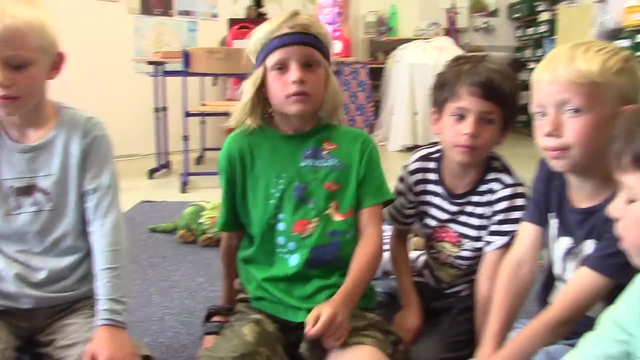 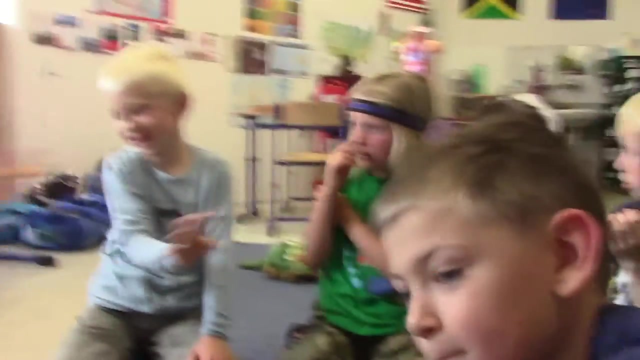 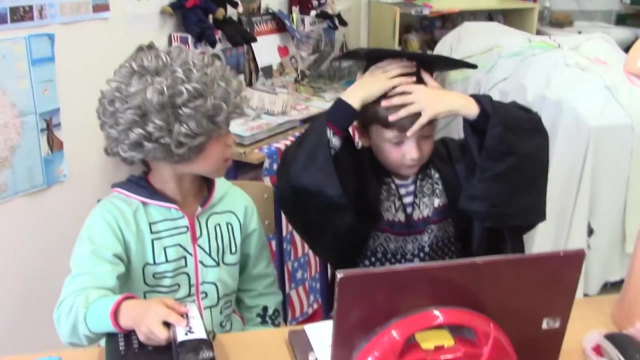 okay, I appreciate that. thanks, thank you very much. I appreciate that. thank you so much, professor Killian. give world, it means, yeah, the professor's. thank you very much. thank you very much for your help. you're welcome and goodbye, no, hello, goodbye, goodbye, goodbye, bye, bye, professors. professors, yes, you can I have. 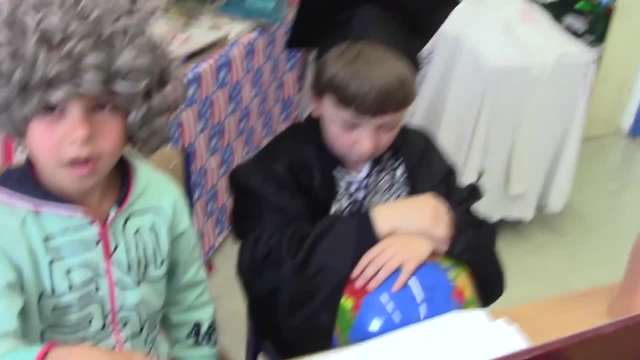 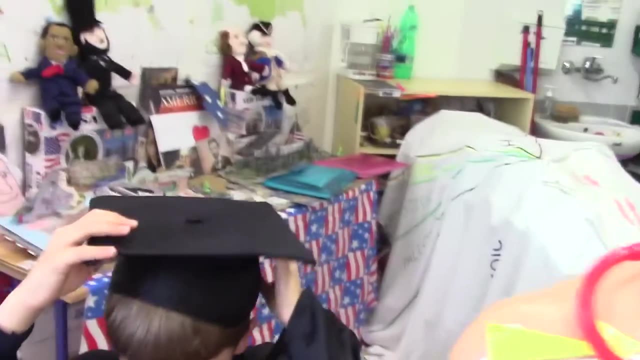 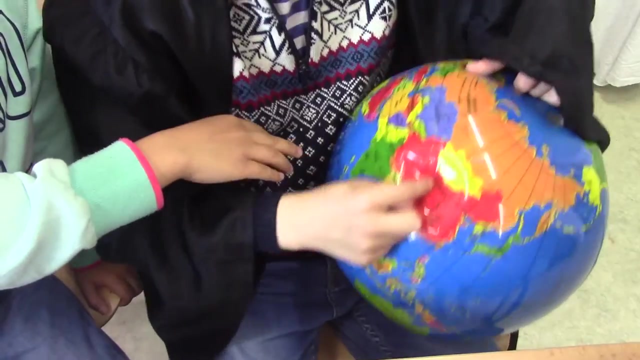 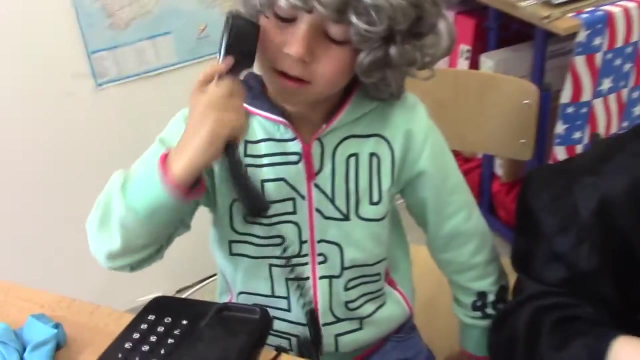 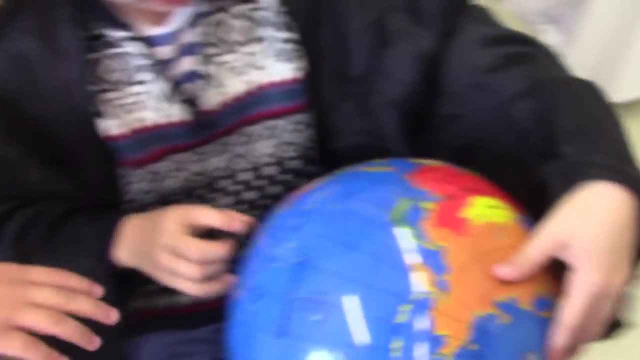 a question for you. I see you're working. I'm sorry, but can I ask one question, one question, okay, where is, where is China? where is China? okay, thank you very much. thank you, that was it, bye, bye, oh, wait, wait, I have a question again. where is Australia? I see, thank you. 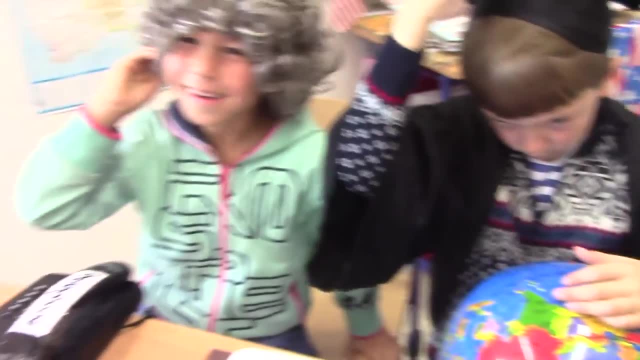 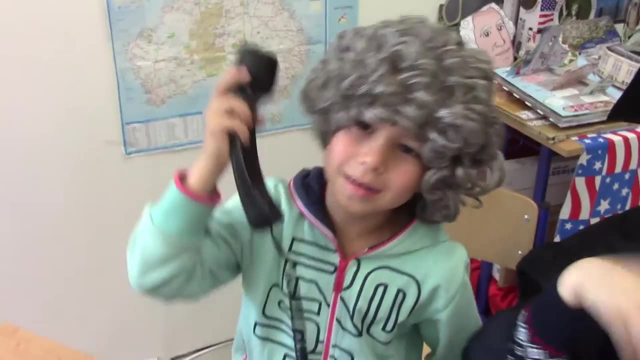 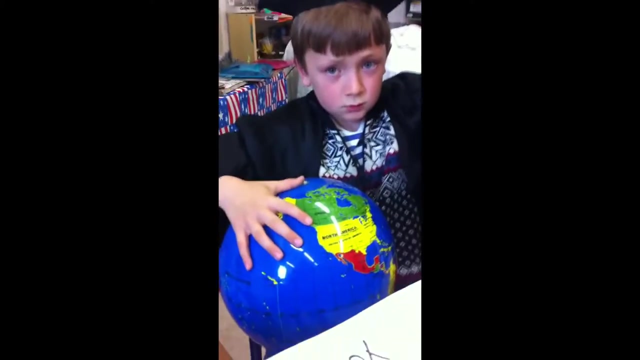 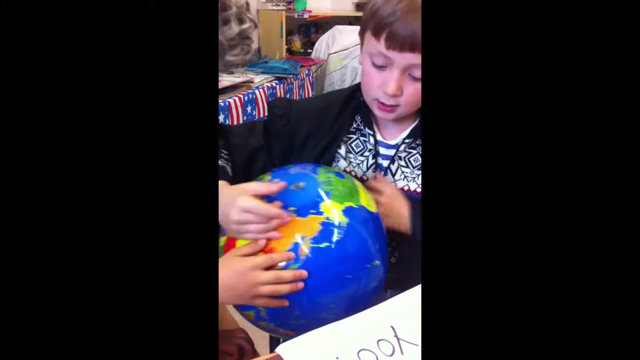 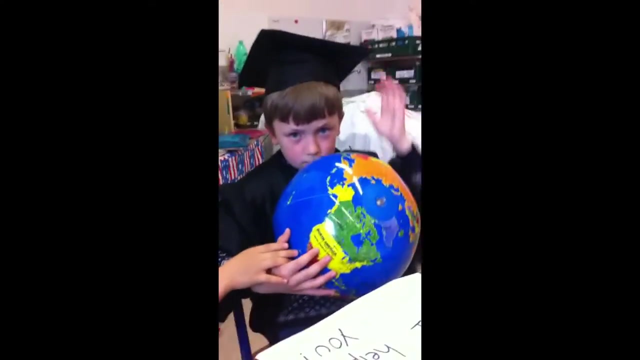 very much, professors, I'm sorry to bother you, I'm sorry. bye, bye, wait, wait, wait. I have another question. I'm sorry, professor. where is? where is United States of America? here's America, I see, and can you show me a professor? I'm sorry to bother you, can you show me?